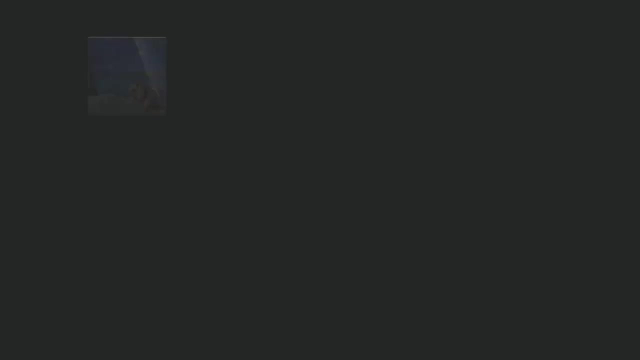 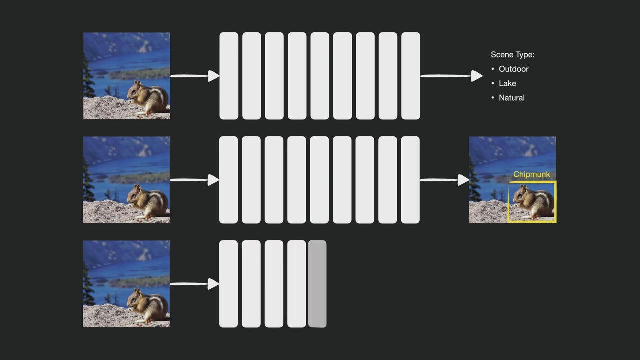 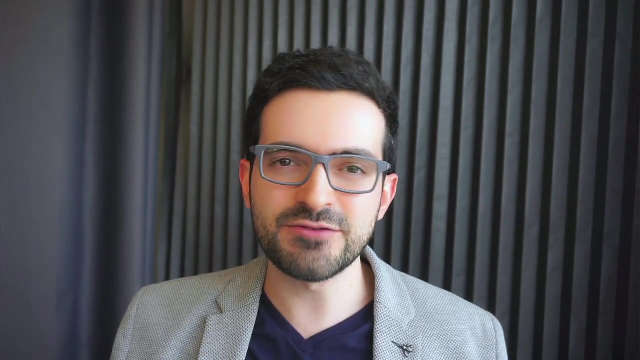 share some of the layers between different but related tasks. For example, if we want to classify a scene, detect objects in it and also output a segmentation mask, do we really need to train three separate models? All these three tasks involve some level of scene understanding. 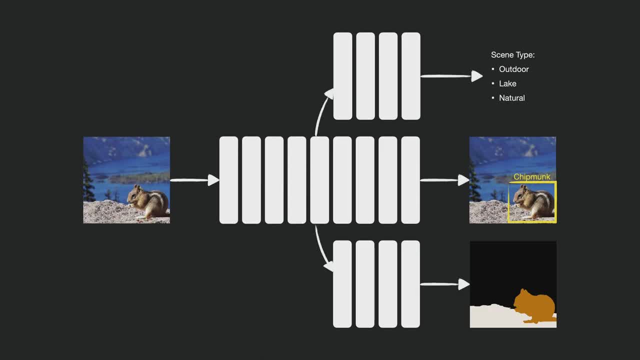 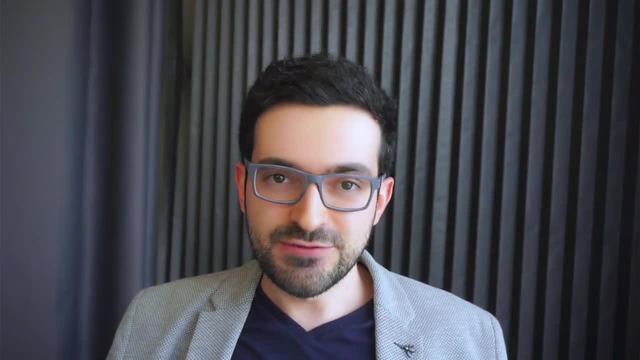 so we could potentially save some memory, computation and power by building a unified multitask. Efficiency is especially important in embedded applications. If you're running your model on low-power devices, any amount of power you can save can make a difference. So how can we do that? 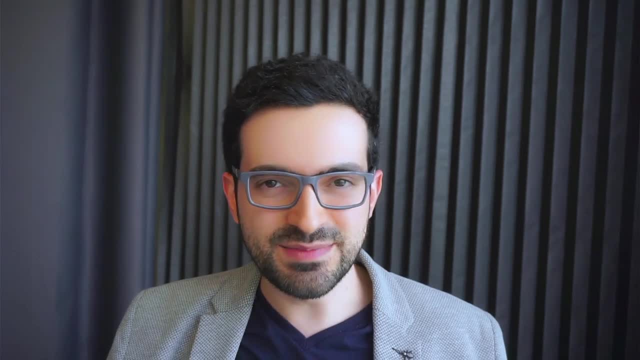 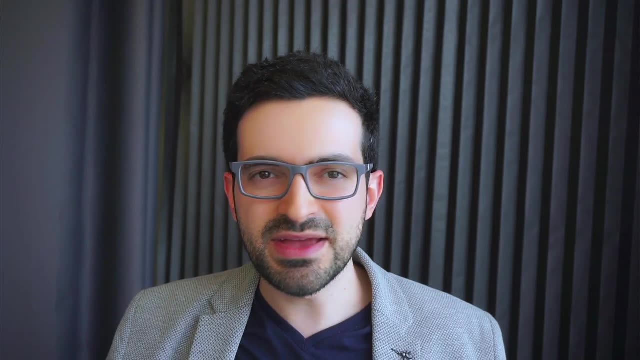 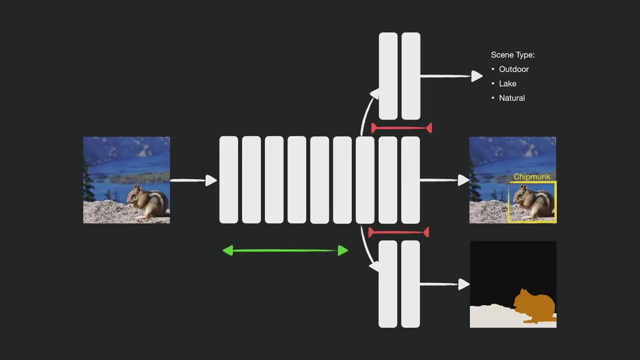 from a model architecture perspective, Perhaps the simplest thing we could do would be to use a shared backbone followed by multiple heads, each dedicated to one task. There are many architectural considerations that we can make here: How much capacity to allocate to the shared backbone, how big the heads should be, where the heads should branch off. 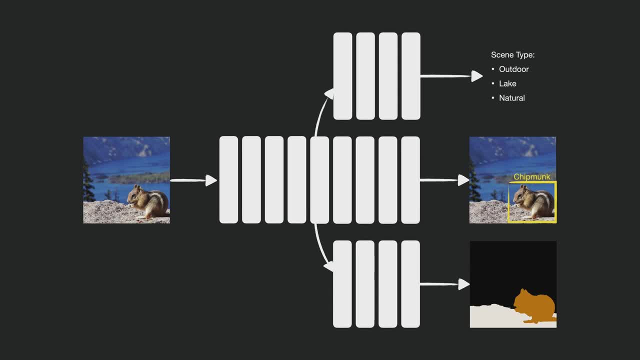 and so on. When we allocate more capacity to the shared part and less capacity to the non-shared part, the tasks are forced to share more features. therefore they become more tightly coupled. Intuitively, the closer the tasks are, the more features they can share. but 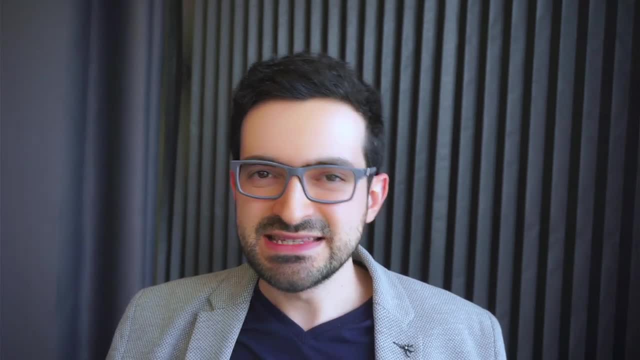 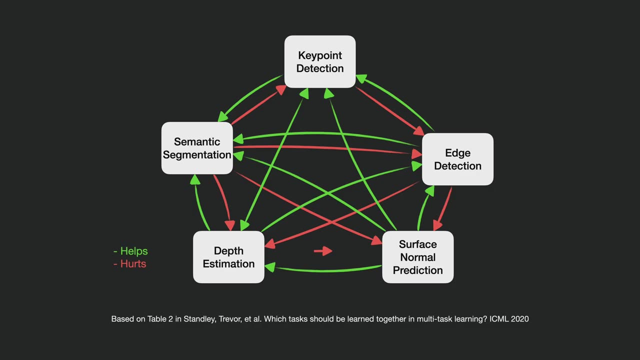 how close the tasks are may not be always straightforward. Seemingly related tasks can hurt each other's accuracy when trained together, so in practice it takes some trial and error to design a multitask model. We don't have to have a hard branching in our architecture. 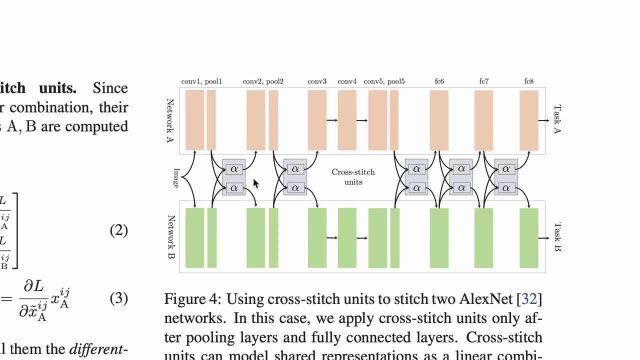 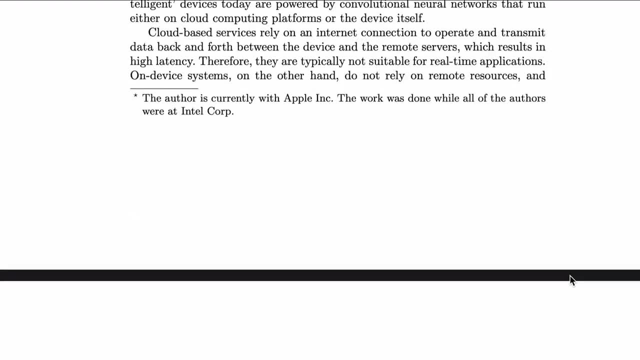 like in the previous example, We can also define soft parameter sharing mechanisms, like the cross-stitch networks from CVPR 2016, or semi-thread-o-nets that I proposed in this ECCV 2020 paper, where how much of the features should be shared is determined by trainable. 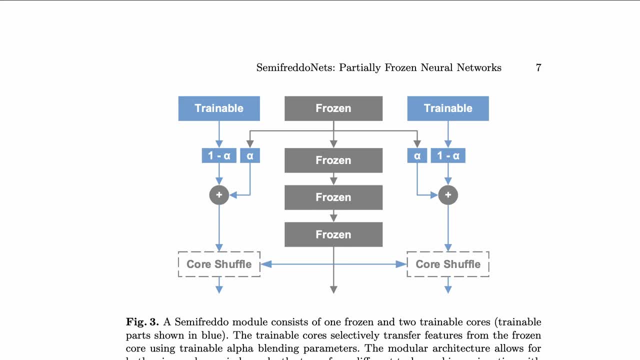 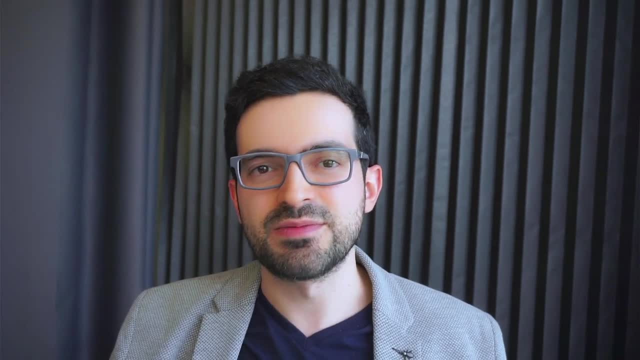 parameters. I'll put the links to the papers in the description. So far we focused only on the efficiency aspect of multitask learning. Efficiency is not the only motivation for multitask learning, though. When done right, learning multiple tasks together can help a model learn a better. 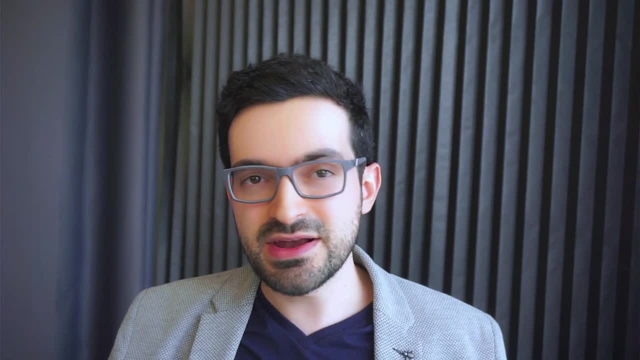 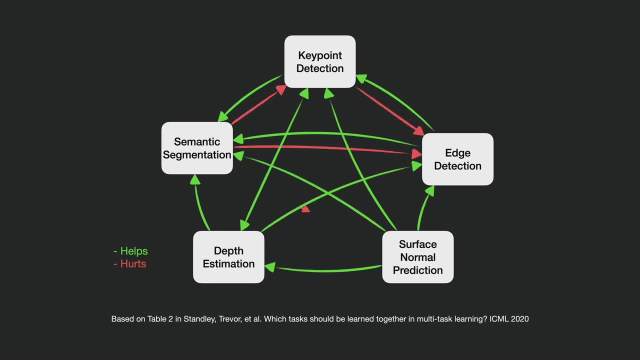 representation and generalize better too. But a better representation is not guaranteed when multiple tasks are learned together. Some tasks help each other, but some others don't get along well. This ICML 2020 paper has some good insights about what tasks should be learned together. 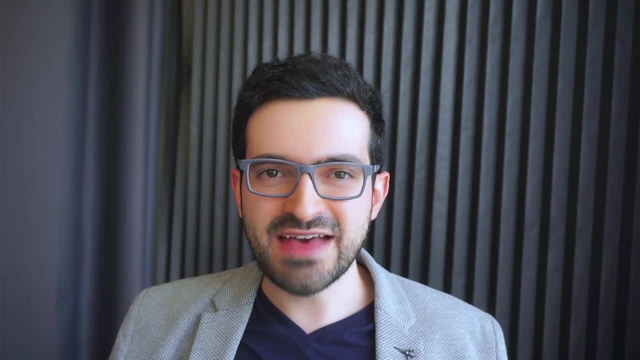 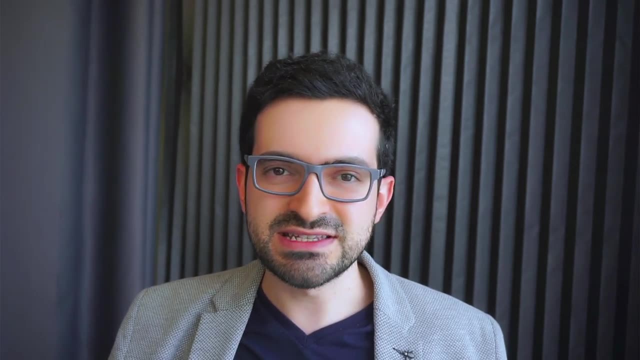 and which ones should not. Alright, let's say we already have a multitask model architecture. To train it, we need to define a loss function and an optimizer. The overall loss function is typically a combination of multiple loss functions corresponding to multiple tasks. How we can combine them depends on a lot of factors. 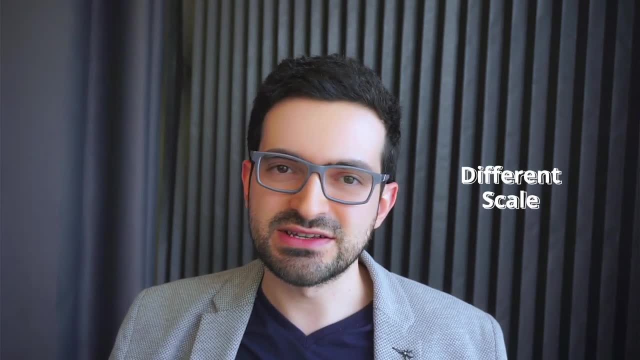 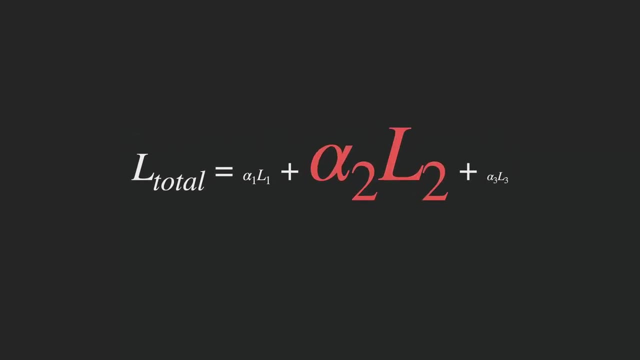 For example, some losses may be on a different scale than others, such as cross-entropy, and mean squared error losses. If one loss is much larger than the others, then it may dominate training. Some losses may be easier to optimize than others. Some losses may be more important to 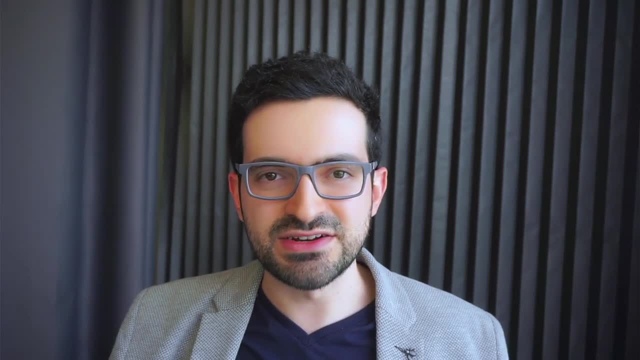 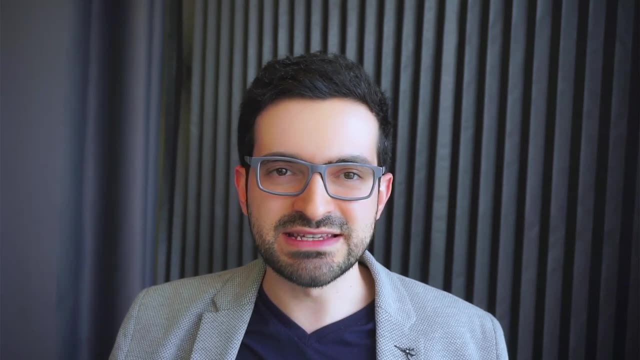 the overall system. Some losses may converge faster than the others, so the relative magnitudes of the weights may be constantly changing. As you can see, assigning weights to each one of these tasks manually can be cumbersome and sometimes outright impossible. Luckily, there are some. 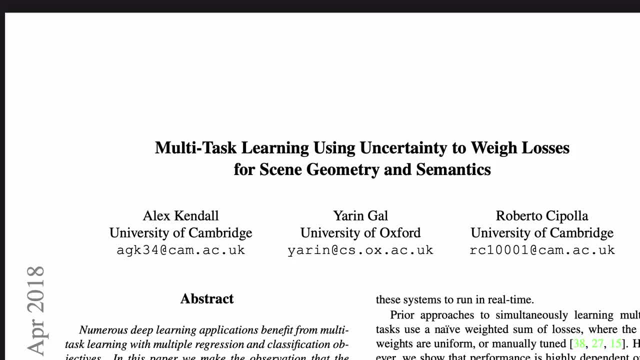 approaches that aim to do that automatically. In this paper titled Multitask Learning: Using Uncertainty to Weigh Losses. for Scene Geometry and Semantics, the authors propose to weigh multiple loss functions by considering the uncertainty of each task. I won't go into the math much, but 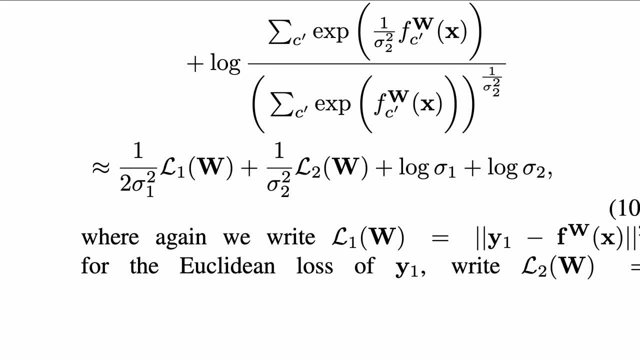 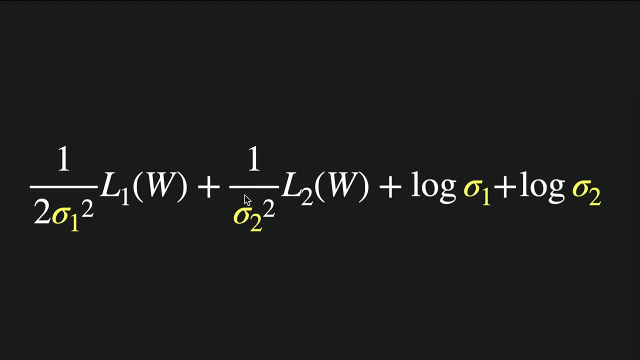 let's take a look at how this combined loss function works intuitively. They basically define these sigmas as trainable parameters for each task. If a task has a higher uncertainty, a larger sigma will decrease its contribution to the overall loss function. The log sigmas here will penalize setting the sigmas unnecessarily large. 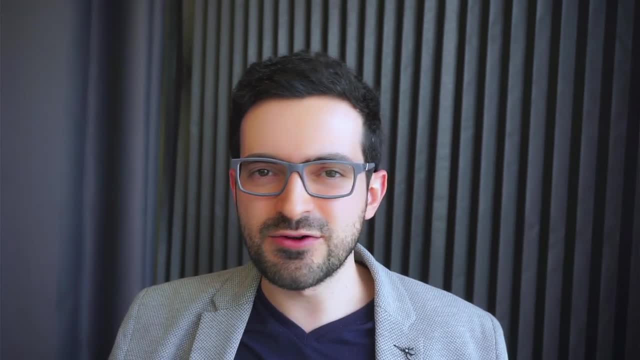 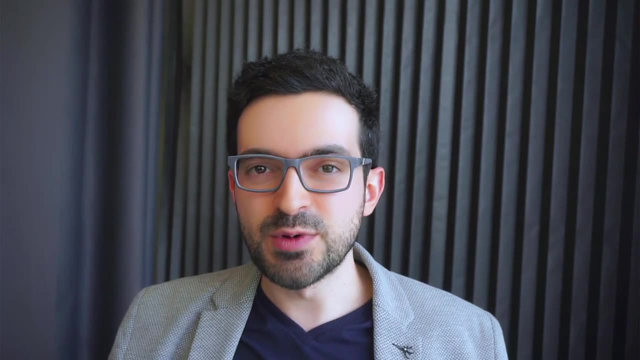 Otherwise, the model can always say: I'm not sure to minimize the overall loss function As the uncertainty goes to the infinity. the loss would go to zero without these additional terms. Another approach to loss balancing is proposed in this paper named Gradnorm. 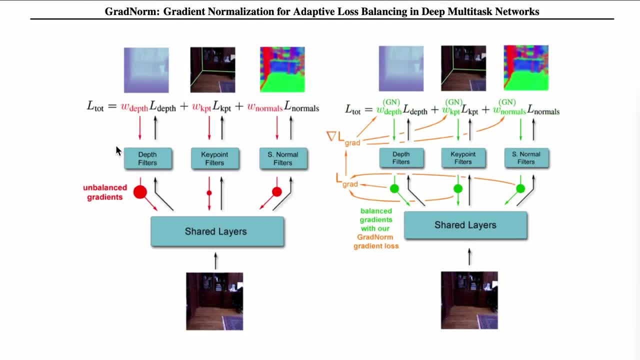 Gradnorm adjusts the weights of the losses in a way that balances the gradient magnitudes. The training is considered balanced when the loss ratio is similar for all tasks and the loss ratio is basically the loss for a given task as compared to its initial value. 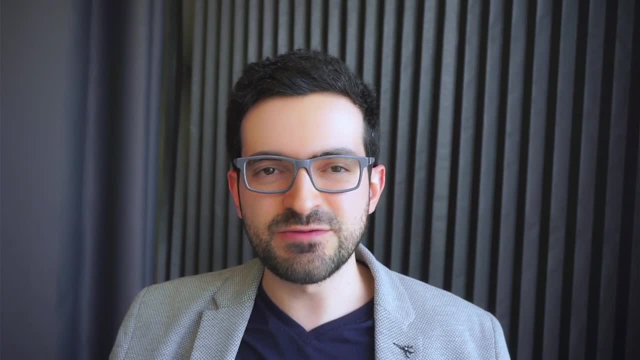 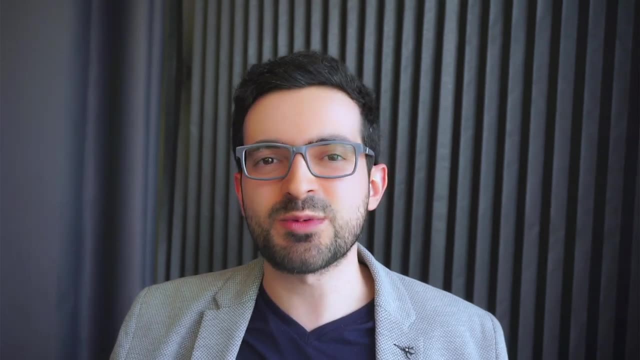 This balanced training setup aims to prevent some tasks from getting too far ahead as compared to others. The idea of Multitask Learning sounds very intuitive and promising, but in practice it doesn't always work well. Sometimes, training a separate model for each task performs better because of the gradient.